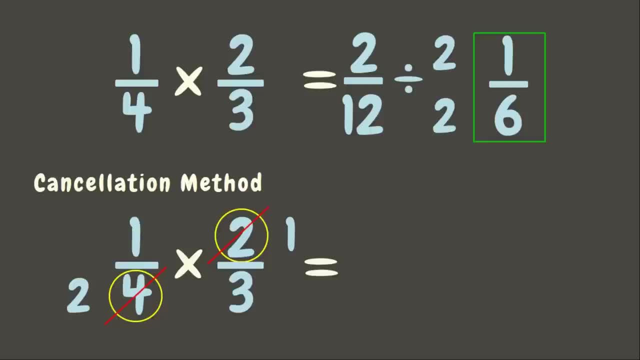 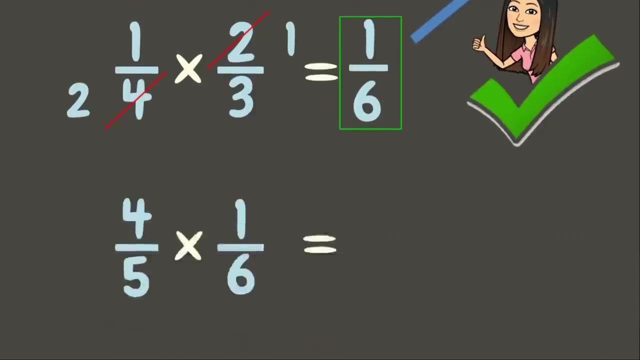 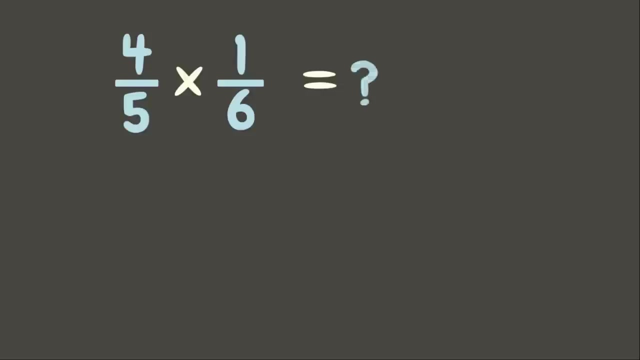 denominator that have common factor. no more, now we can multiply the numerators and denominators: 1 times 1 is 1. 2 times 3 is 6. now our answer is 1- 6. awesome, now let us try another example: 4, 5 times 1, 6. 4 times 1 is 4. 5 times 6 is 30. now let's. 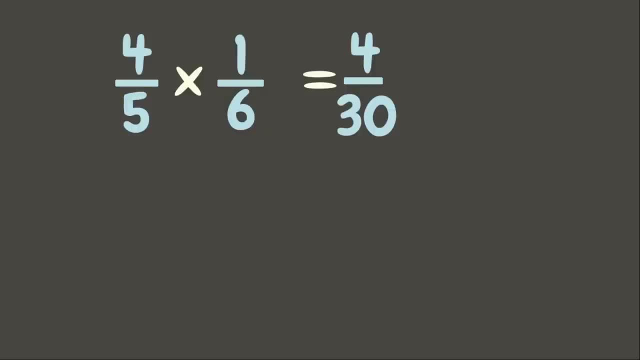 simplify our answer: 4 and 30 can be divided by its common factor 2: 4 divided by 2 is 2, 30 divided by by 2 is 50. factor 2: 4 divided by 2 is 2. 30 divided by 2 is 50. 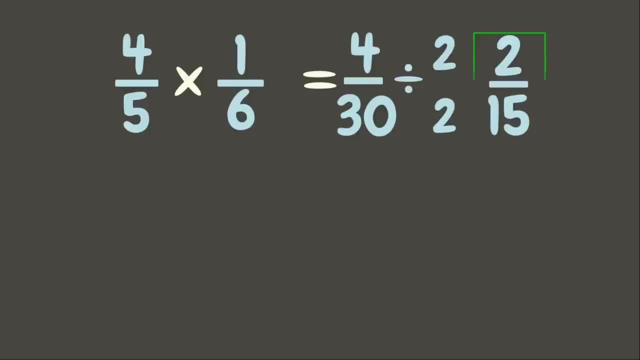 factor 2- 4 divided by 2 is 2- 30. divided by 2 is 50. our final answer is 2- 15 now. our final answer is 2- 15 now. our final answer is 2- 15 now. let us try cancellation method. 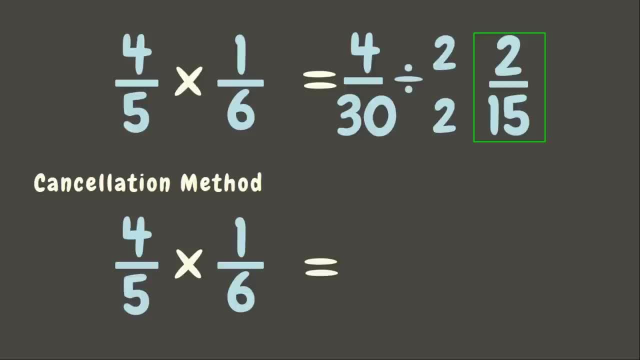 now, let us try cancellation method. now, let us try cancellation method. now can you find a numerator? and now can you find a numerator. and now can you find a numerator and denominator which have common factor. denominator which have common factor. denominator which have common factor. very good, 4 and 6 have common factor of. 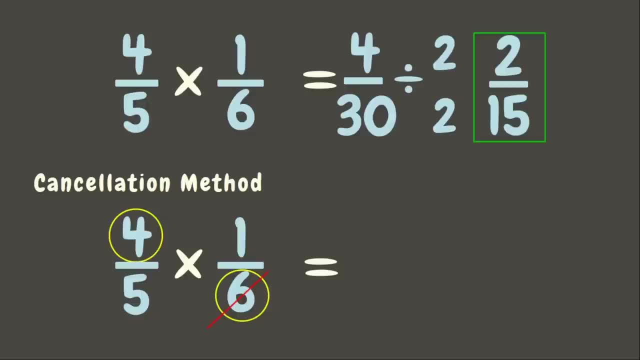 very good. 4 and 6 have common factor of very good. 4 and 6 have common factor of 2. now let us divide them by 2. 6 divided 2. now let us divide them by 2. 6 divided 2. now let us divide them by 2, 6 divided by. 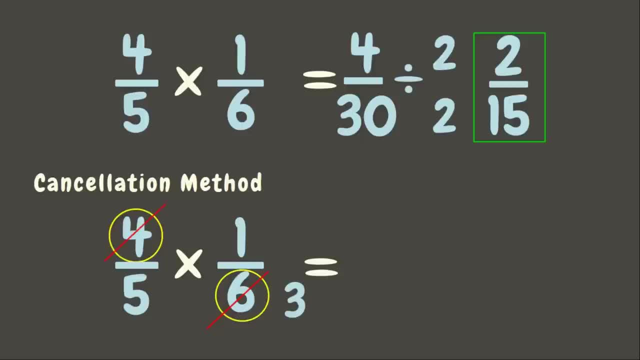 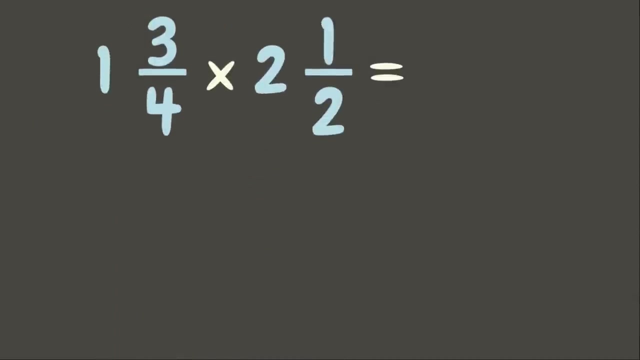 by by 2 is 3, while 4 divided 5 by 2 is 2. now let's multiply them: 2 times 1 is 2. 5 times 3 is 15. now we got the same answer. now, this time we are going to multiply mixed numbers. in multiplying mixed, 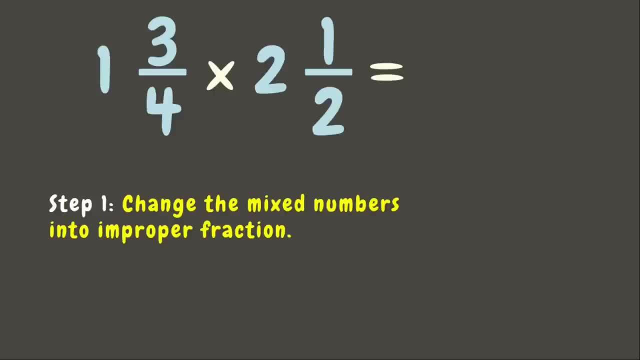 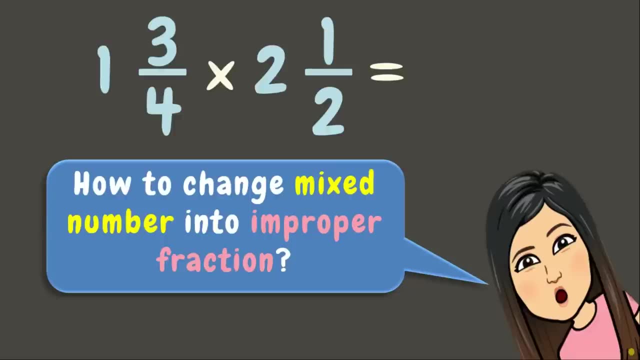 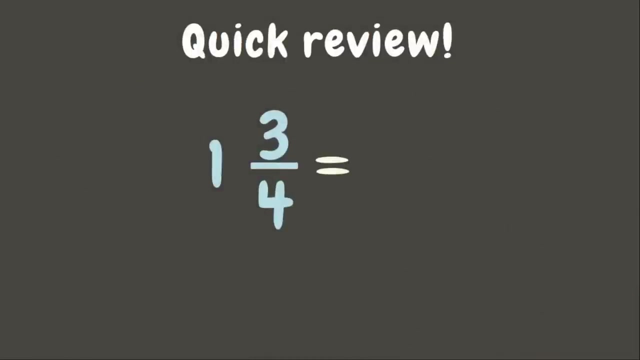 numbers. we need to change them into improper fraction. but how are we going to change the mixed number into improper fraction? let's have a quick review. to change mixed number into improper fraction, we multiply denominator to the whole number 4 times 1 is 4 and then add it into. 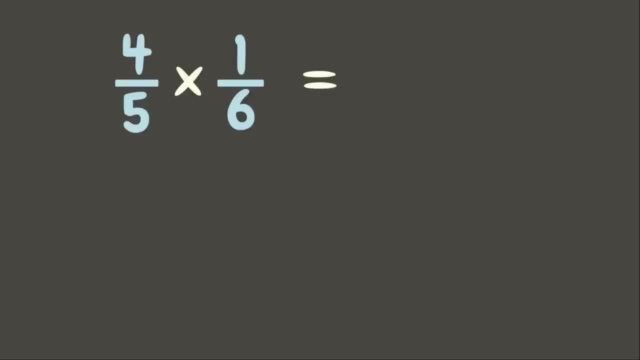 Six times one-sixth. Four times one is four. Five times six is thirty. Now let us simplify our answer. Four and thirty can be divided by its common factor two. Four divided by two is two. Thirty divided by two is fifteen. Our final answer is two-fifteenths. 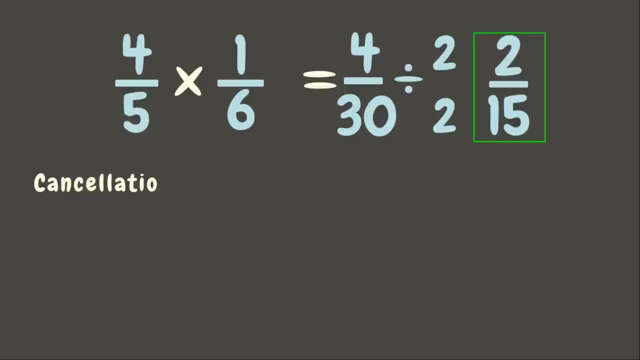 Now let us try cancellation method. Now can you find a numerator and denominator which have common factor? Very good, Four and six have common factor of two. Now let us divide them by two. Six divided by five, by two is three, While four 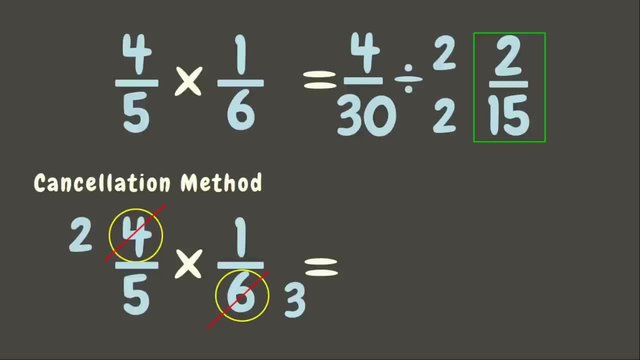 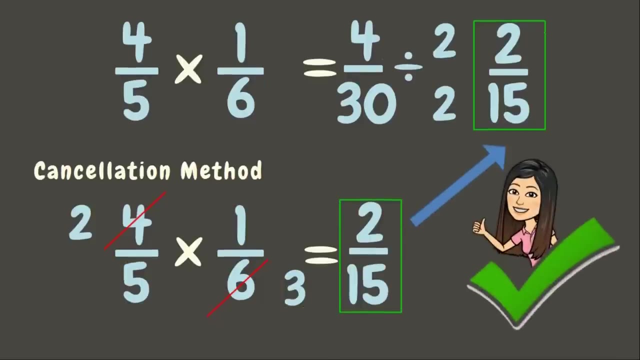 divided by five by two is one. Now let us try calculation method. Three divided by five by two is from: Five divided by five by three is eight. ThisALW слово, kiwayat, is showed in the Korean English language Because five divided by five by two is two. Now let us multiply them Two times: one is two. 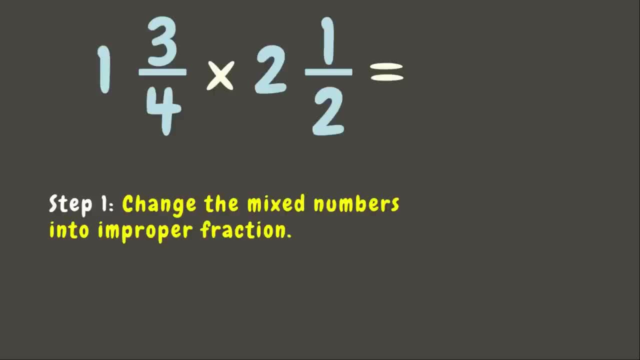 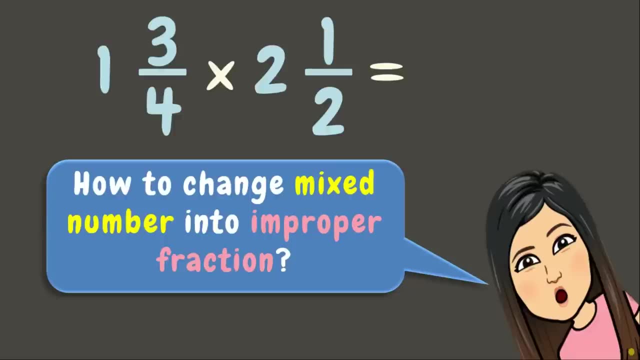 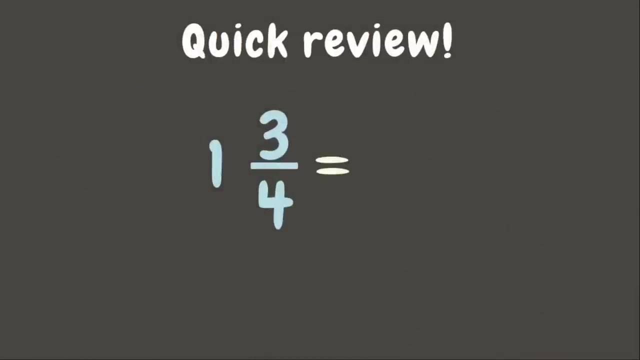 five times three is fifteen them into improper fraction. But how are we going to change mixed number into improper fraction? Let's have a quick review. To change mixed number into improper fraction, we multiply denominator to the whole number 4 times 1 is 4.. And then add it into the numerator Plus 3 is 7.. And then we 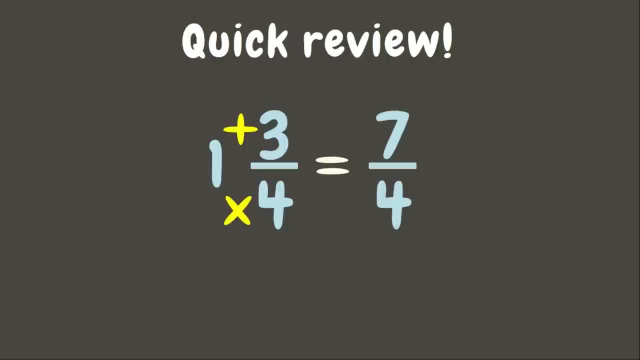 simply copy the denominator 4.. Now, 1 and 3 fourths is equivalent to improper fraction 7 fourths. All right, Now let's go back. Let's change each mixed number into improper fraction 4 times 1 is 4.. Plus 3 is 7. Over 4. Next. 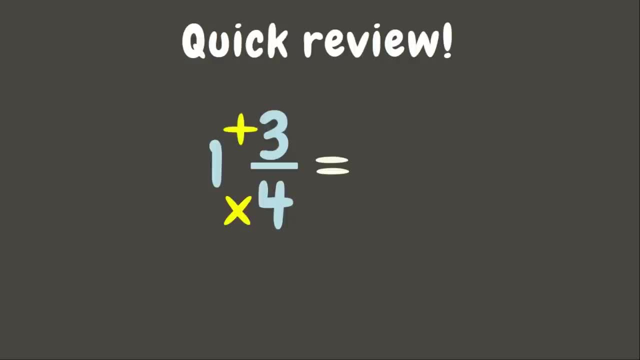 the numerator plus 3 is 7.. And then we simply copy the denominator 4.. Now, 1 and 3 4ths is equivalent to improper fraction 7 4ths. Alright, now let's go back. Let's change each mixed. 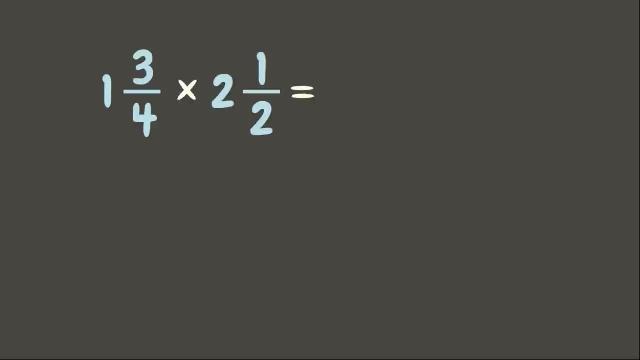 number into improper fraction: 4 times 1 is 4 plus 3 is 7 over 4.. Next, 2 times 2 is 4 plus 1 is 5 over 2.. Now we can multiply them 7 times 5 is 35.. 4 times 2 is 5.. And then: 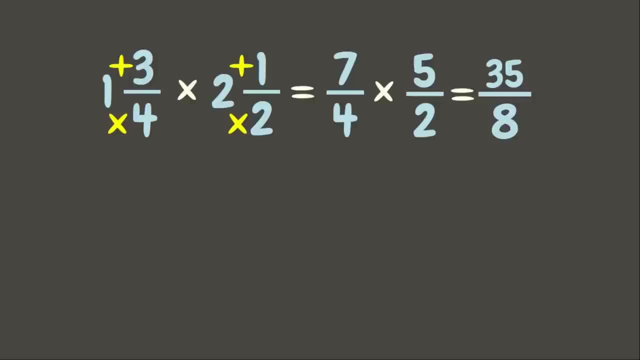 2 is 8.. Now look, our answer is in its improper form. We are going to simplify it by converting it into a mixed number: 35 divided by 8.. 4.. 4 times 8 is 32.. 35 minus 32 is 3.. Now our 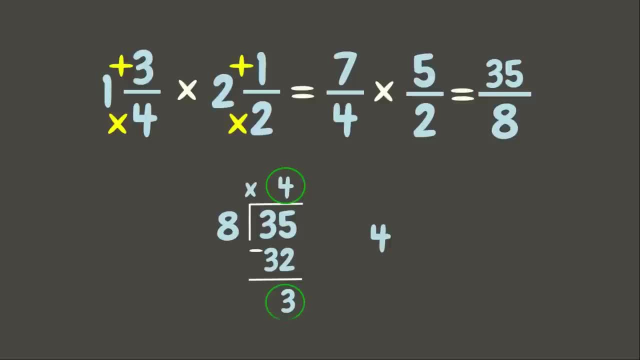 answer is 4 and 3.. And 3 8ths. Now let's have another example. First step: change the mixed numbers into improper fraction. 3 times 1 is 3 plus 1 is 4 over 3.. 5 times 1 is 5 plus 2 is 7 over 3.. 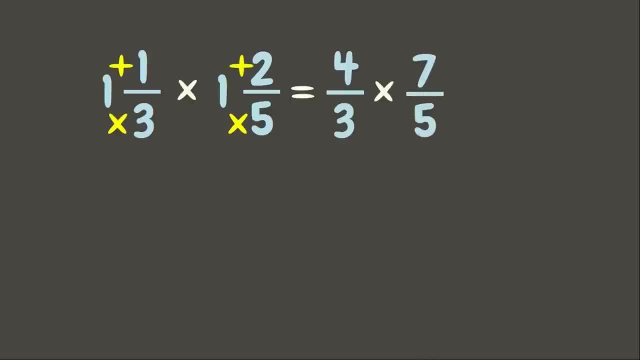 7. Copy the denominator. Now let's multiply: 4 times 7 is 28.. 3 times 5 is 15.. Since it is an improper fraction, we need to change it into mixed number: 28 divided by 15 is 1.. 1. 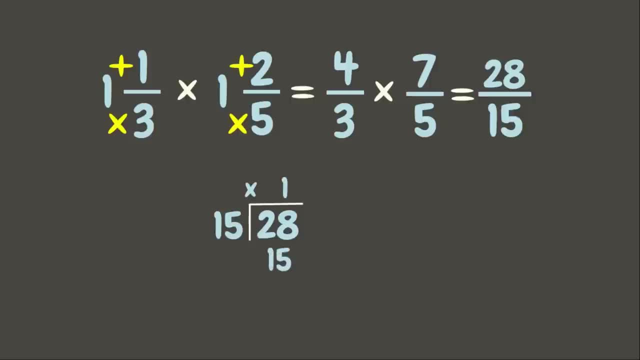 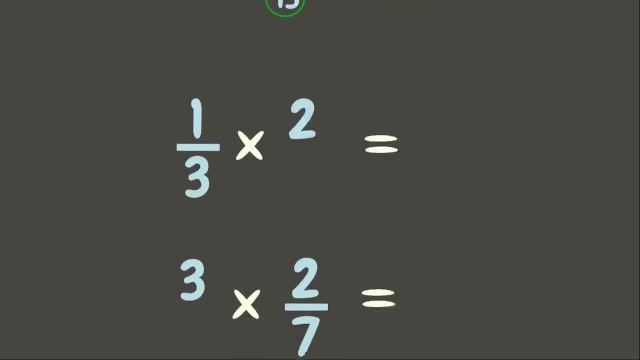 times 15 is 15.. 28 minus 15 is 15.. For the purpose of this fraction In HolaCosmos, we'll explain how to calculate our mixed number in the next video, 13.. Now, our final answer is 1 and 13 15ths. Awesome. Now let us multiply fraction into: 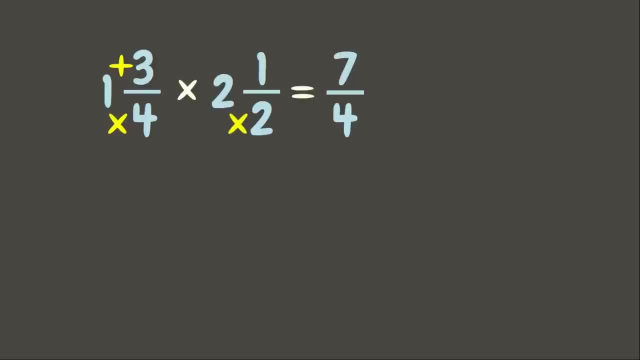 2 times 2 is 4.. Plus 1 is 5.. Over 2.. Now we can multiply them 7 times 5 is 35.. 4 times 2 is 8.. Now look, Our answer is in its improper form. 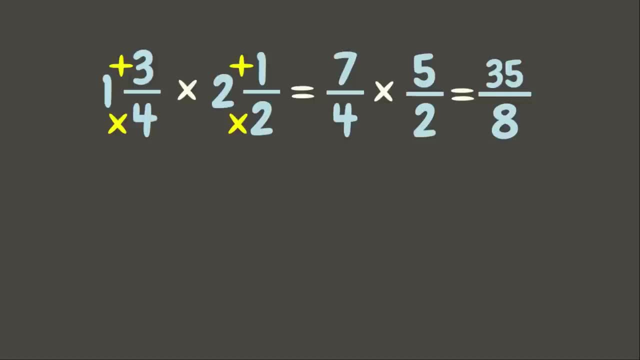 We are going to simplify it by converting it into a mixed number: 35 divided by 8.. 4. 4 times 8., 32.. 35 minus 32 is 3.. Now our answer is: 4 times 2 is 8.. 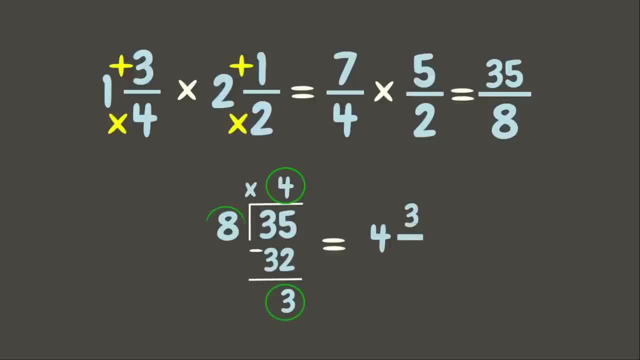 And three-eighths. Now let's have another example. First step: change the mixed numbers into improper fraction. Three times one is three plus one is four over three. Okay, five times one is five plus two is seven. Copy the denominator five. 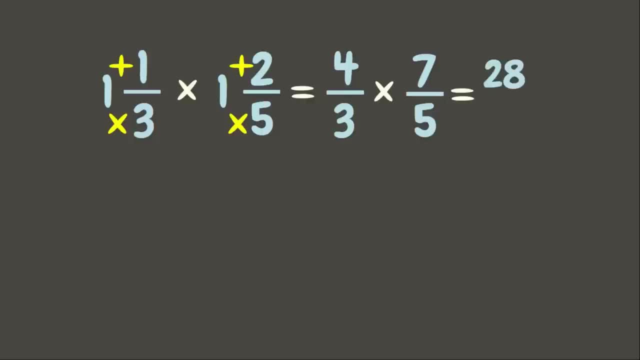 Now let us multiply: Four times seven is twenty-eight. Three times five is fifteen. Since it is an improper fraction, we need to change it into mixed number. Twenty-eight divided by fifteen, Fifteen is one. One times fifteen is fifteen. 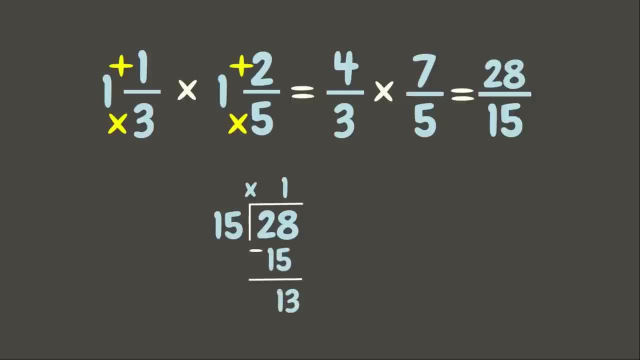 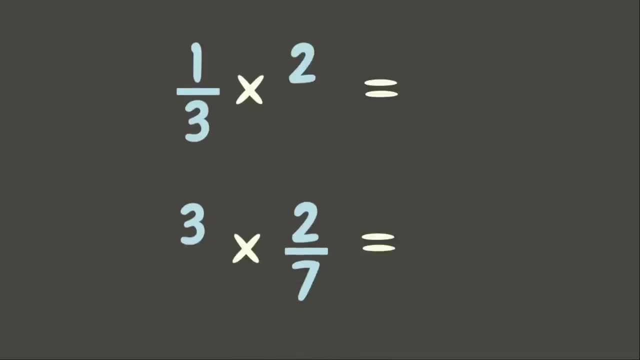 Twenty-eight minus fifteen is thirteen. Now our final answer is one and thirteen-fifteenths. Awesome. Now let us multiply fraction into whole number. In multiplying fraction into whole number, we are going to put one As the denominator of the whole number. 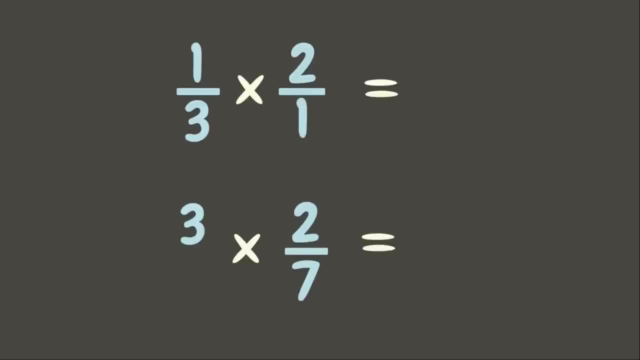 And then simply multiply them: One times two is two, Three times one is three, And that is our final answer. Let's have another example: Three times two-sevenths. Again, let us put one as the denominator of three.